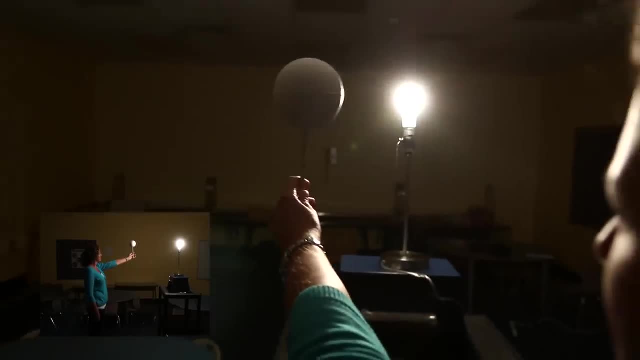 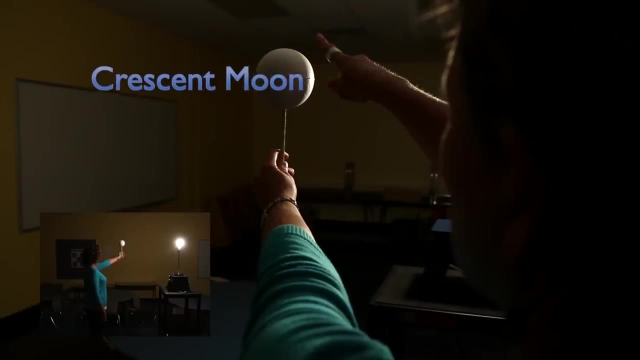 and we can't see the Moon. It's there, but the side that's reflecting sunlight is away from us. Now, as I slowly make the Moon orbit to my left, I can begin to see a tiny sliver of that lighted side. We call that a crescent Moon. As the Moon keeps orbiting, we can see. 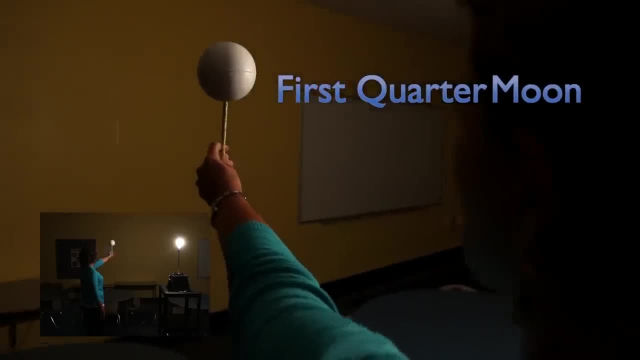 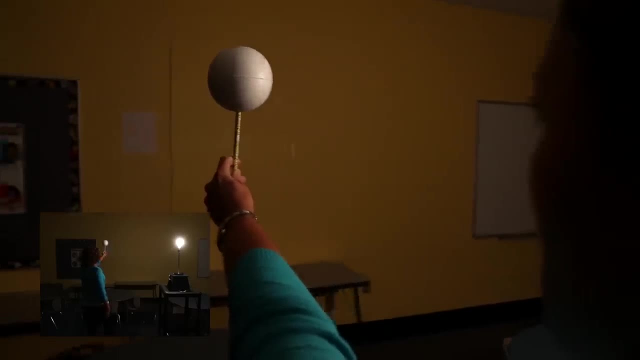 more and more of that lighted side. We see half of the lighted half, which is a quarter Moon, In this case a first quarter Moon. Subtitles by the Amaraorg community. As we keep orbiting, we see almost the whole lighted side. We call that a gibbous Moon. 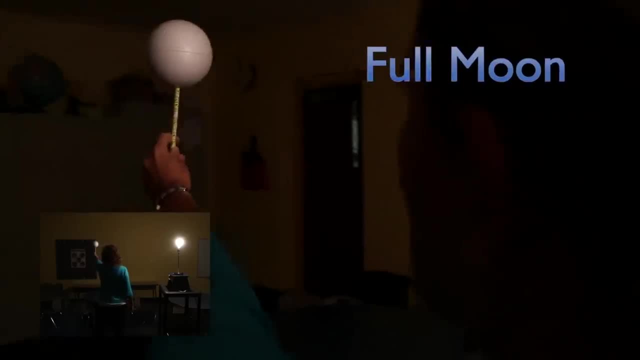 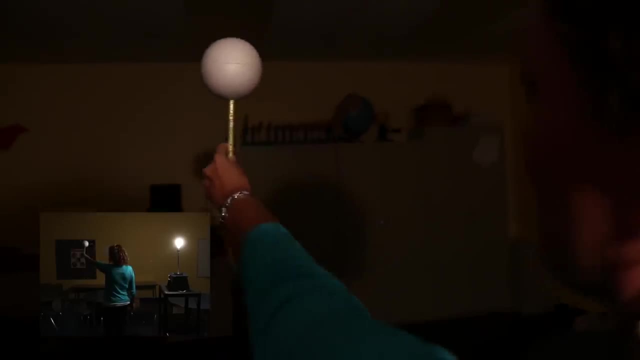 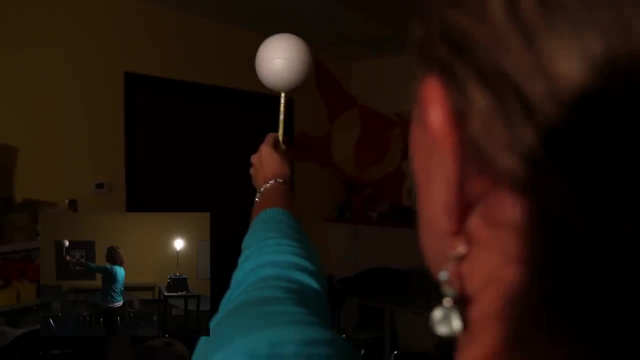 Then, when we can see the entire lighted half of the Moon, that's a full Moon. As the Moon continues in its orbit, we begin to see less and less of that lighted side. We're back to a gibbous Moon, but this time the light is on the opposite side. 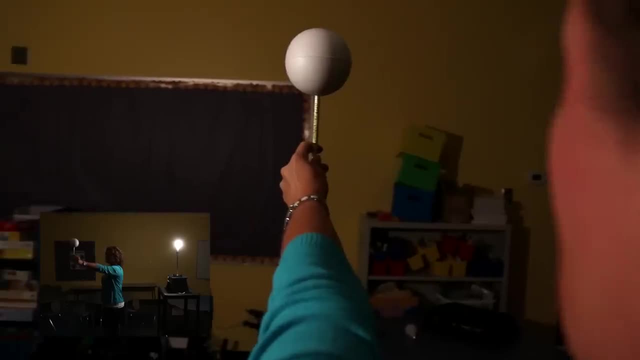 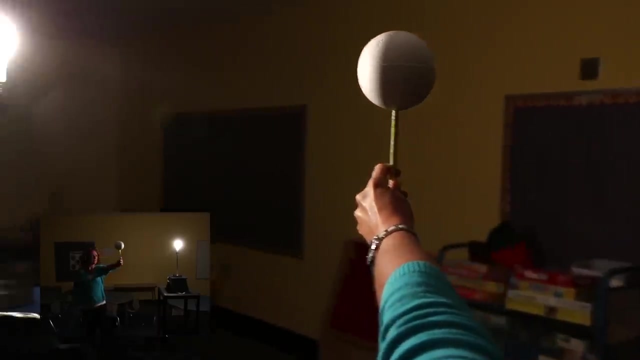 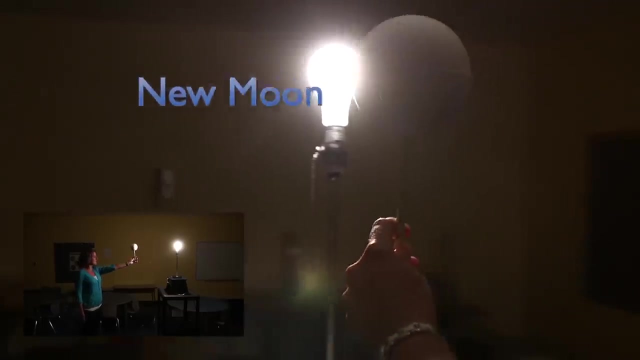 Subtitles by the Amaraorg community. Yet another quarter Moon, or last quarter Moon, to be exact. Subtitles by the Amaraorg community. Another crescent, a percent of sun And finally back to New Moon And the cycle begins again. 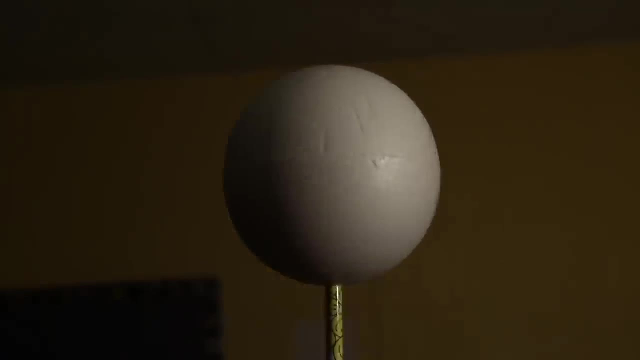 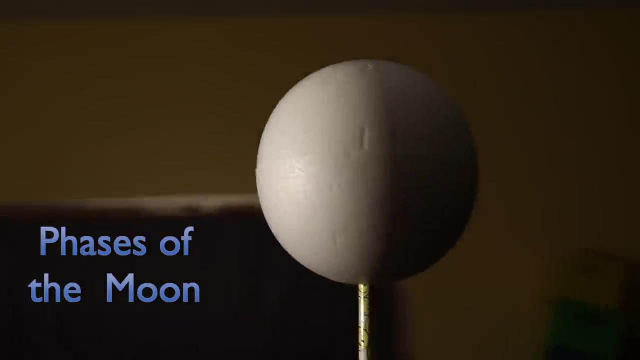 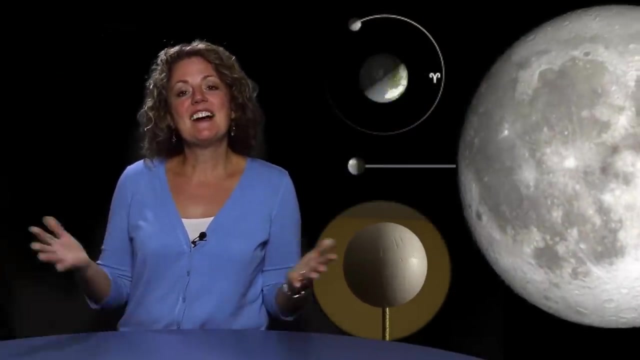 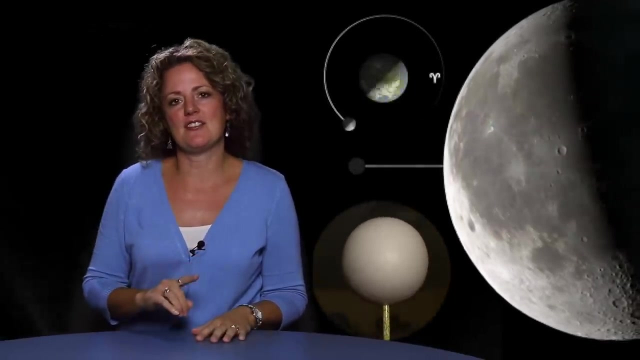 Watching bola bouncing off that green slope. Now it is proper for life to rest, so it doesn't Origin in hell and a spring storm on Mars. So why does the moon appear in different shapes throughout the month? Because of its orbit. The shape or phase of the moon depends on where it is in its orbit around Earth. 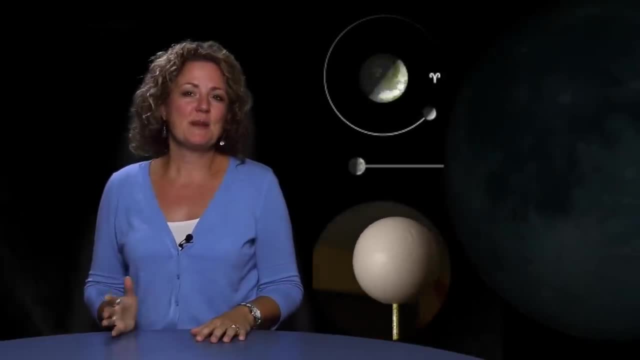 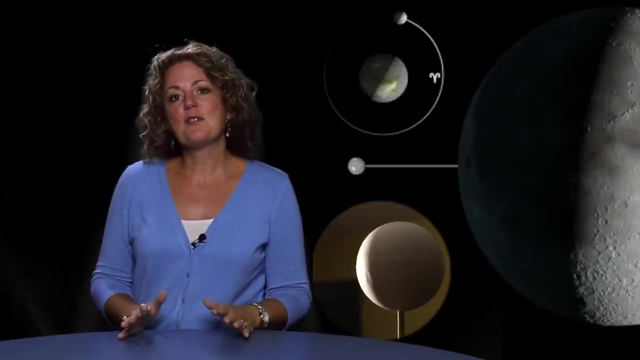 It takes about a month for the moon to orbit the Earth, So when you look up at the moon today, know that you'll see that same phase again about a month from now. Thank you for watching and I hope you give this activity a try. 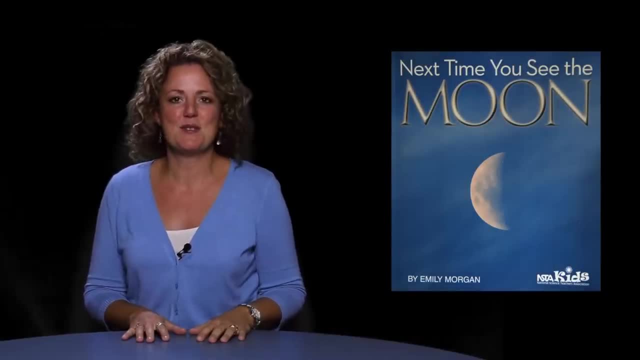 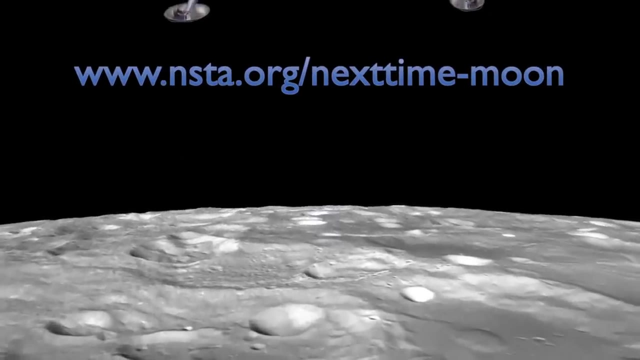 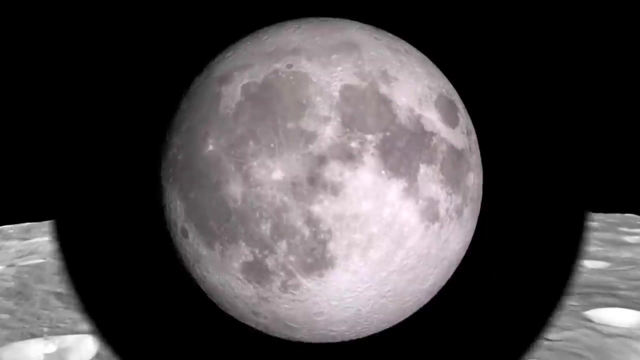 And I hope that you have a sense of wonder next time you see the moon. For a full description of this activity and other resources for teaching about moon phases, go to wwwnstaorg. slash next time dash moon. There are moon calendars and other science and reading activities there. 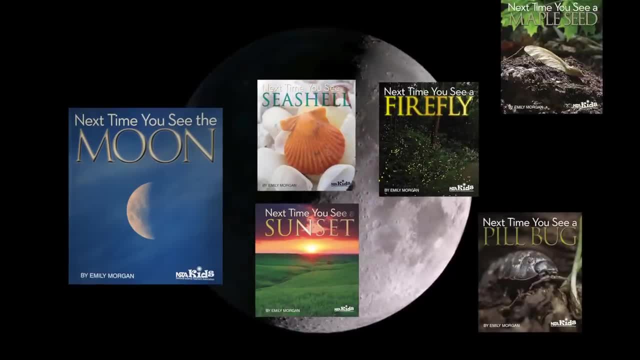 For more information about the Next Time You See book series, visit wwwnexttimeyouseeorg. That's nexttimeyouseecom. 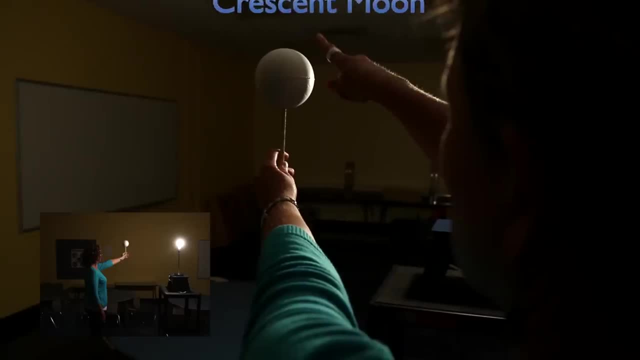 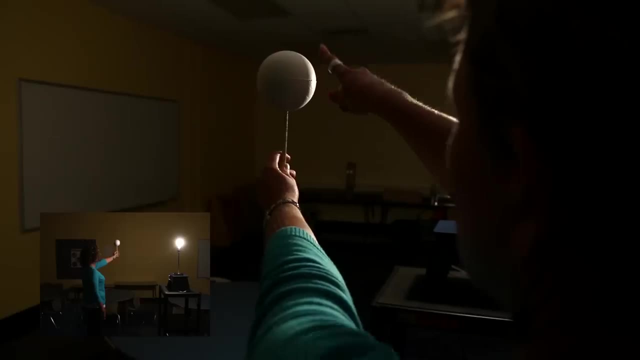 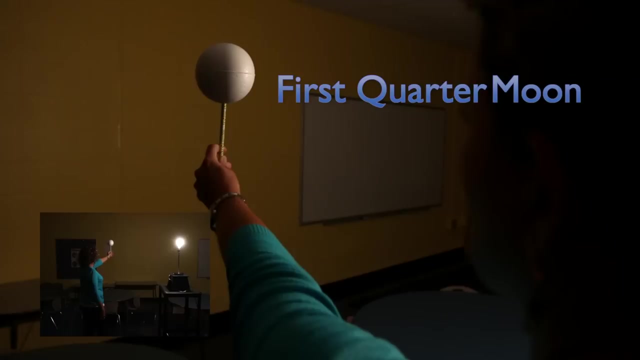 away from us. Now, as I slowly make the moon orbit to my left, I can begin to see a tiny sliver of that lighted side. We call that a crescent moon. As the moon keeps orbiting, we can see more and more of that lighted side. We see half of the lighted half, which is a 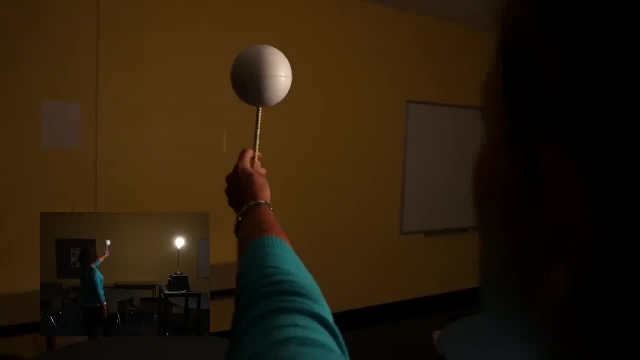 quarter moon, In this case a first quarter moon. E Bereich Malhab Hal. respuesta 1ust. we see half of the lighted half, which is a quarter moon, In this case A first quarter moon moon. As we keep orbiting, we see almost the whole lighted side. 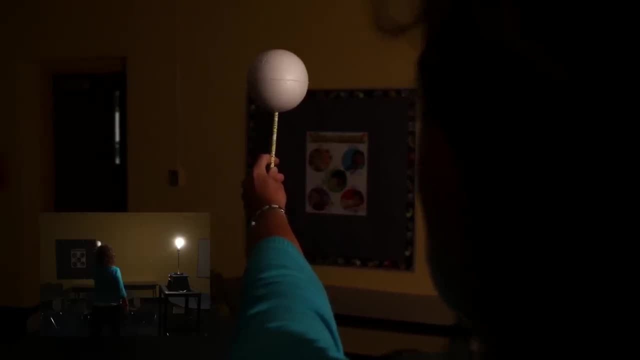 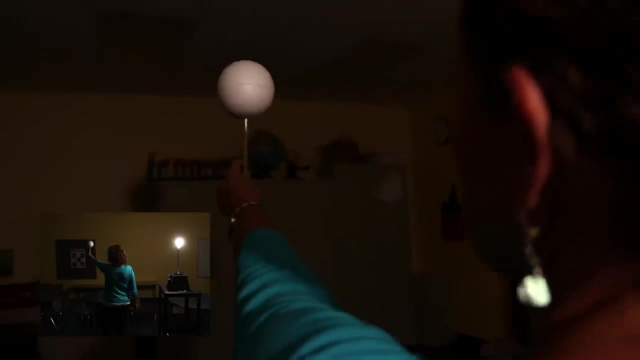 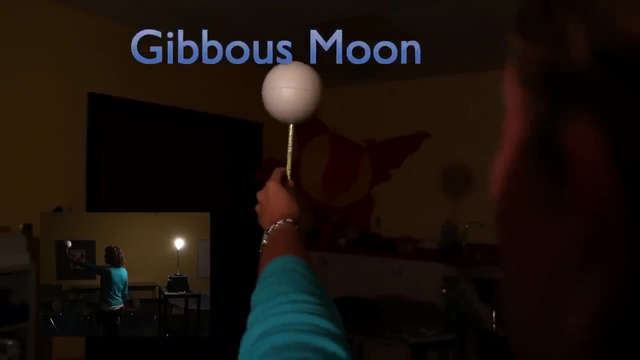 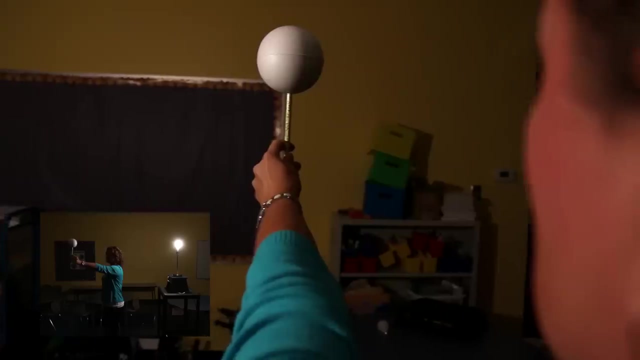 We call that a gibbous moon. Then, when we can see the entire lighted half of the moon, that's a full moon. As the moon continues in its orbit, we begin to see less and less of that lighted side. We're back to a gibbous moon, but this time the light is on the opposite side. 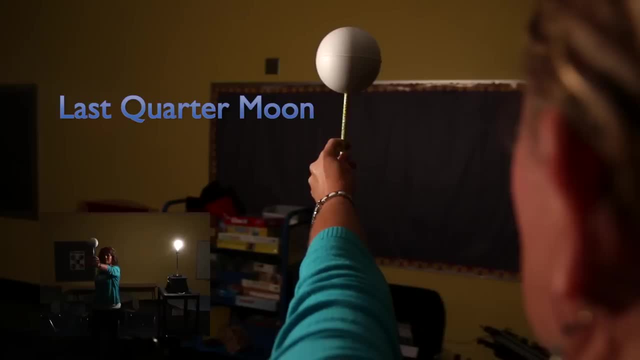 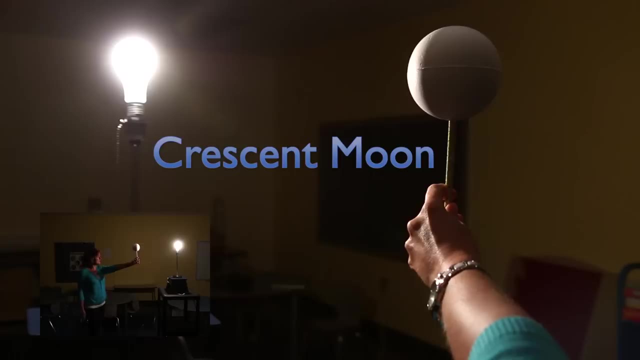 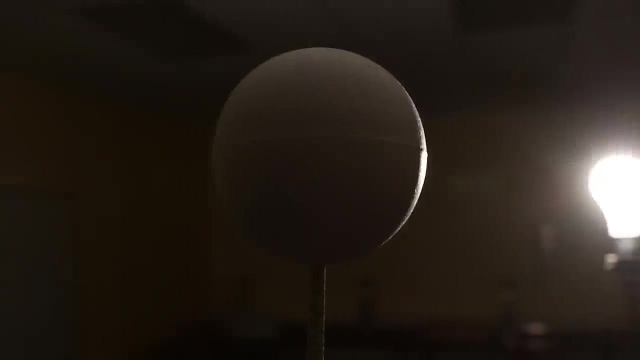 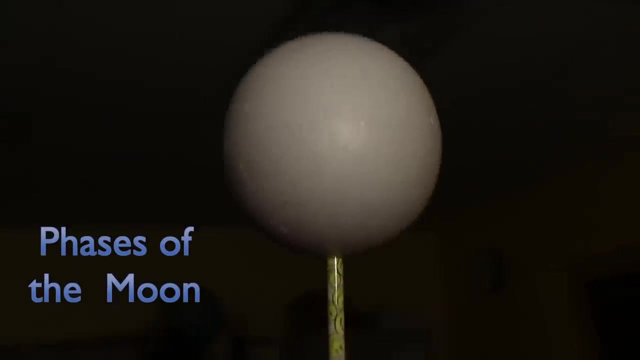 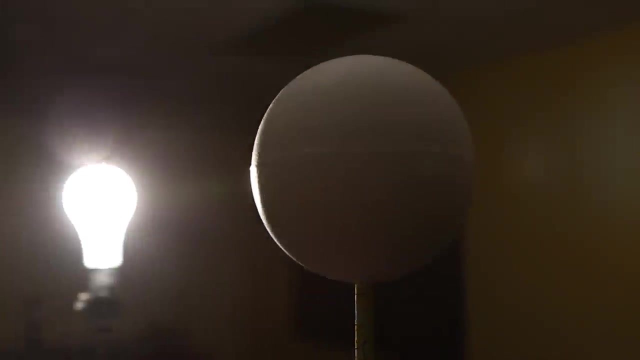 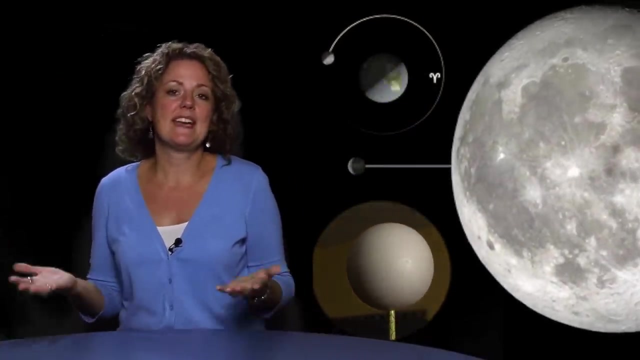 Then another quarter moon- last quarter moon, to be exact- Another crescent And finally back to new moon And the cycle begins again. Okay, So why does the moon appear in different shapes throughout the month? Because of its orbit. The shape or phase of the moon depends on where it is in its orbit around Earth. 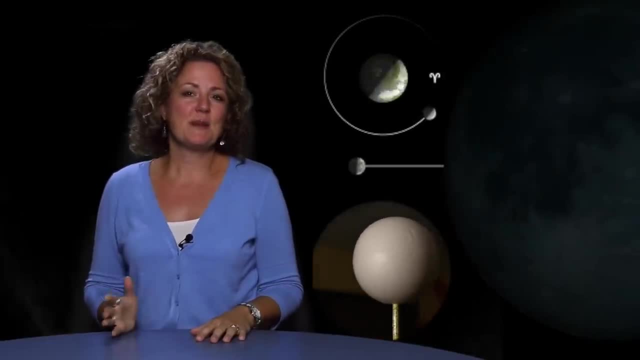 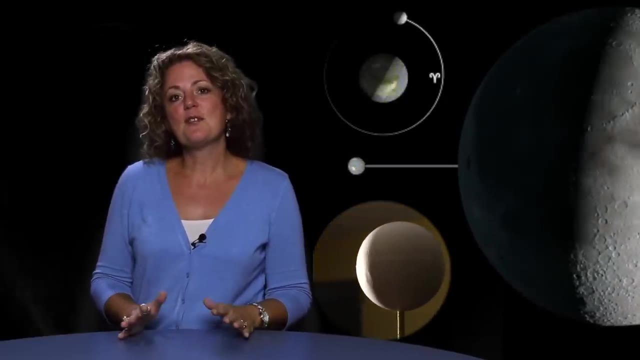 It takes about a month for the moon to orbit the Earth, So when you look up at the moon today, Know that you'll see that same phase again about a month from now. Thank you for watching and I hope you give this activity a try, and I hope that you have. 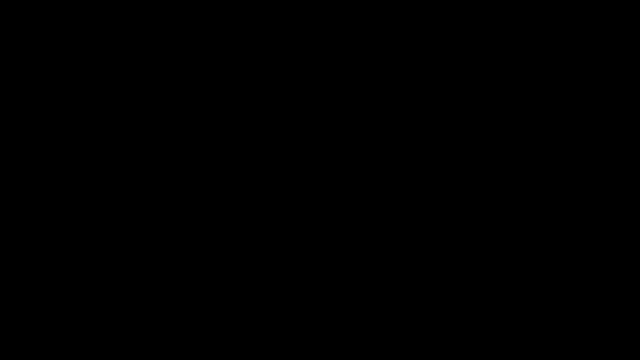 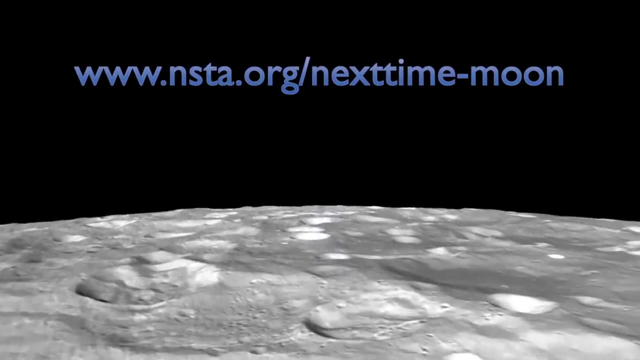 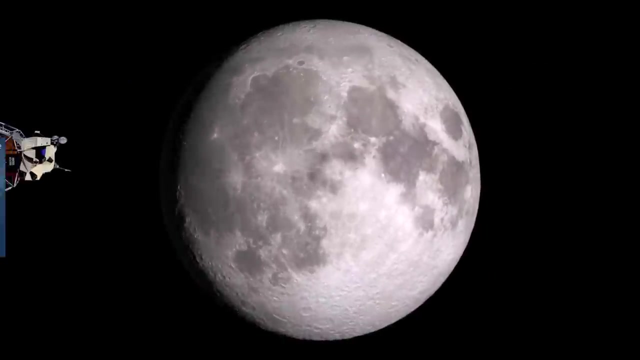 a sense of wonder next time you see the moon. For a full description of this activity and other resources for teaching about moon phases, go to wwwnstaorg. slash: next time dash moon. There are moon calendars and other science and reading activities there. 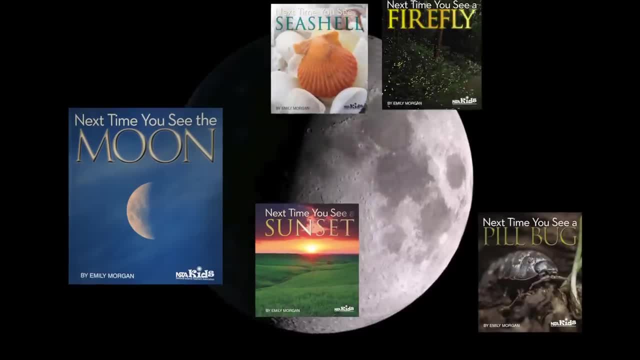 There are moon calendars for littoral objects and moon survey. hare, hahaha, 你BEER. But if you meet a head for a moon that just got out of town, this video is for you. For more information about the Next Time You See book series, visit wwwnexttimeuccom.